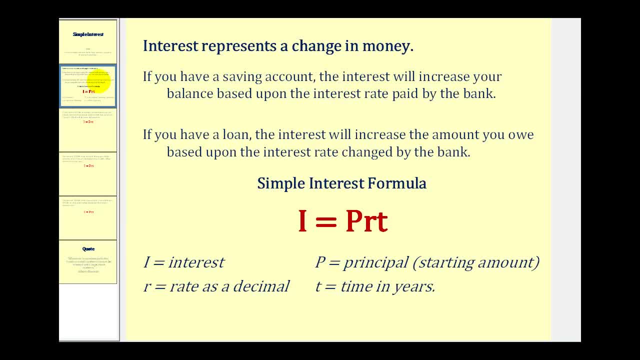 the earnings on an investment or savings account or how interest will affect how you pay back a loan. Interest represents a change in money, So if you have a savings account or investment account, interest will increase your balance based upon the interest rate paid by the bank, And if you have a loan, the interest. 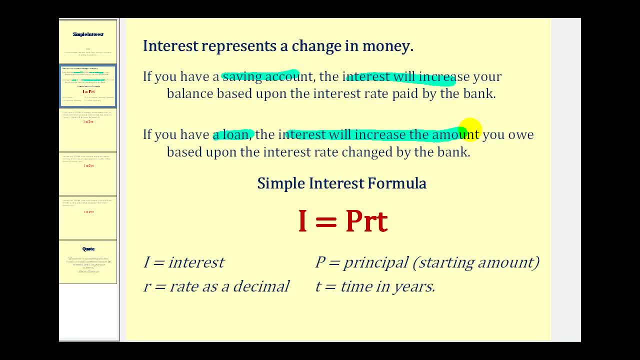 will increase the amount you owe based upon the interest rate charged by the bank. The simple interest formula is: I equals P times R times T. Where I is the interest, P is the principal or starting amount, R is the rate expressed as a decimal. 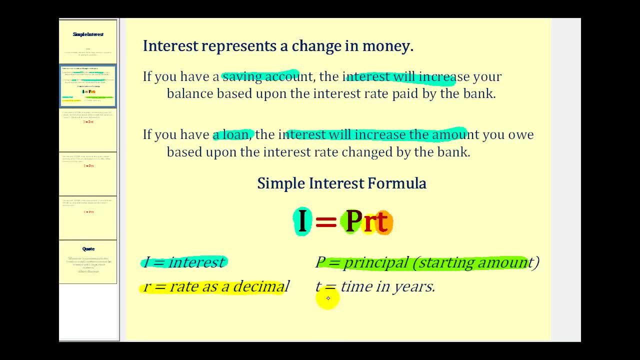 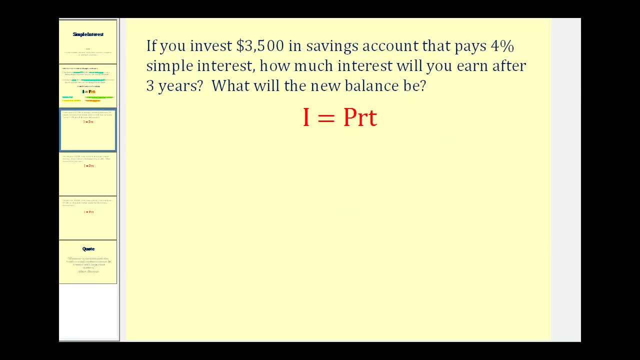 And T is time expressed in years. Let's go and take a look at some examples. If you invest $3,500 in a savings account that pays 4% simple interest, how much interest will you earn after three years and what will the new balance be? So for: 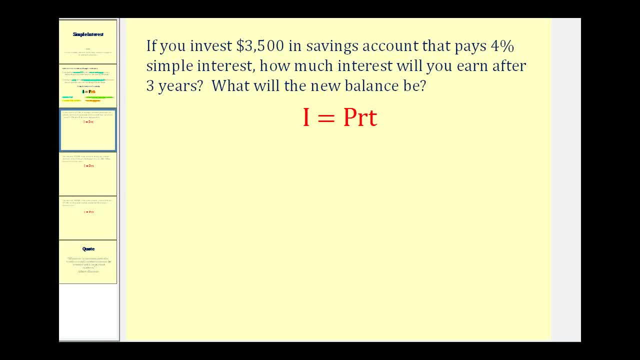 this situation we're trying to find I, or the interest P. the principal or starting amount would be $3,500.. R is the rate of return, So R is 4%, But it must be expressed as a decimal, So this would be 0.04.. And then T is time in. 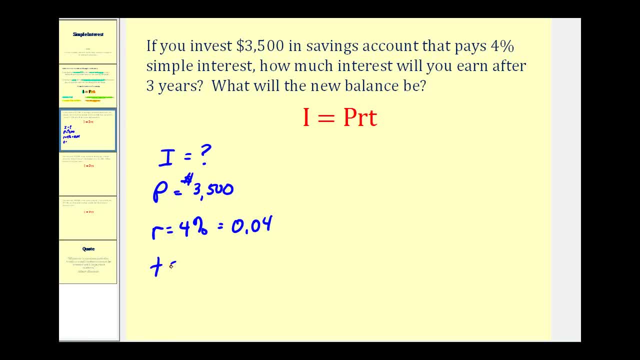 years, So T is equal to three years. We have all the information we need to be able to determine the amount of interest that's earned in this account. The interest will equal $3,500, the principal times the rate of return as a decimal. 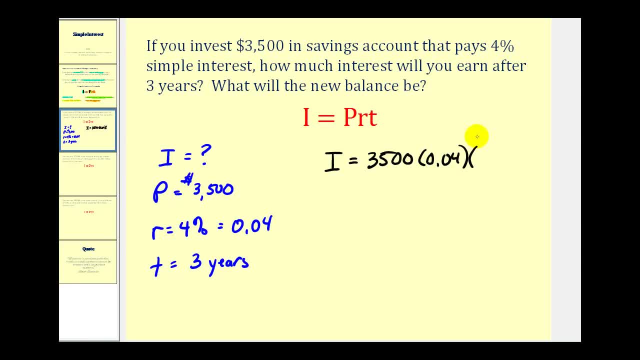 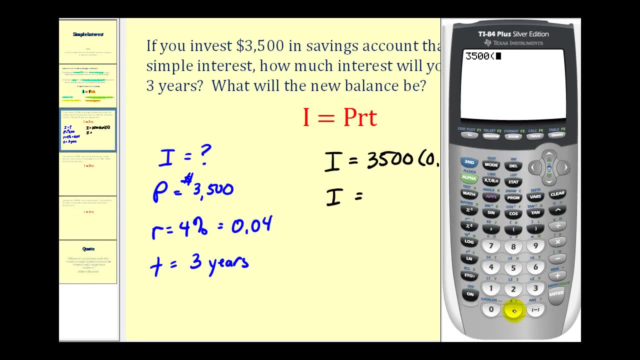 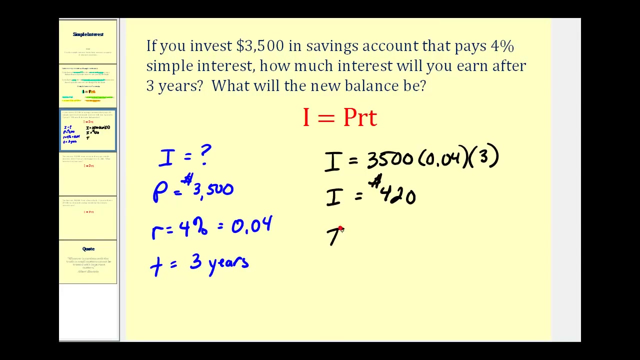 0.04 times the time in years, which is equal to three. So this product will give us our total interest over the three years. So we have $3,500.. Times 0.04 times three, So the interest earned will be $420.. 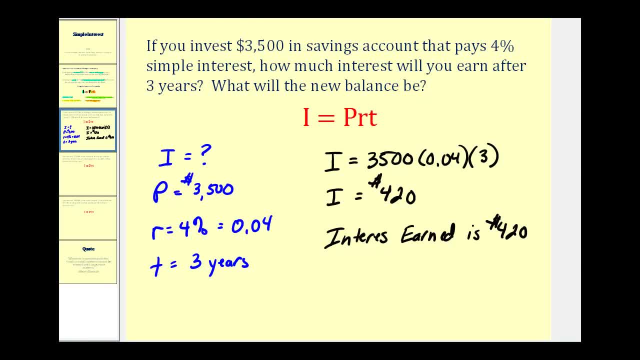 But they also ask us what the new balance of the account will be. So we take our starting amount, 3,500.. And so this, The interest, represents the increase in the balance. so we add $420, and so the ending balance will be $3,920. 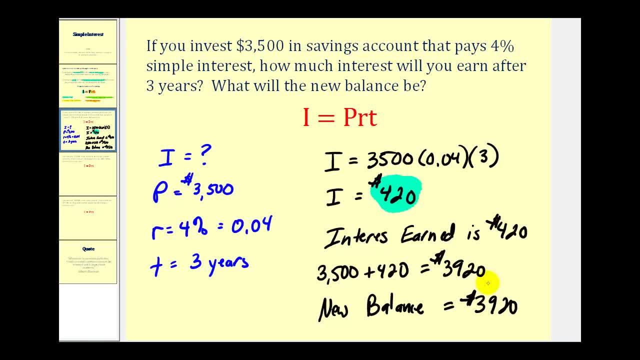 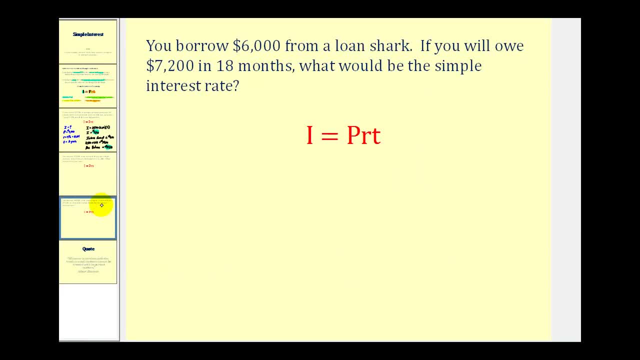 So again we found the interest earned, and then we also found the new balance of the savings account after three years. Let's go and take a look at another example. You borrow $6,000 from a loan shark If you will owe $7,200 in 18 months. 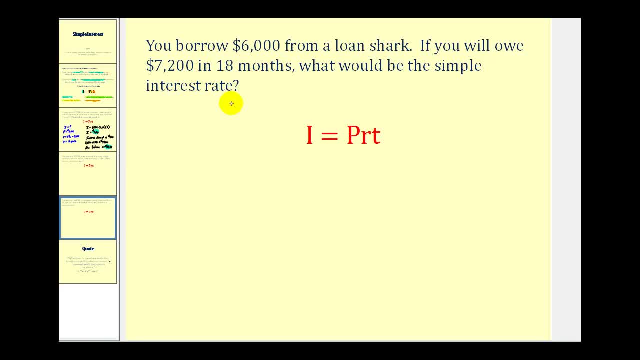 what would be the simple interest rate. So now we're trying to find the interest rate or R, so we should be able to determine I, P and T. Let's see if we can do that. Remember, I represents the amount of interest. 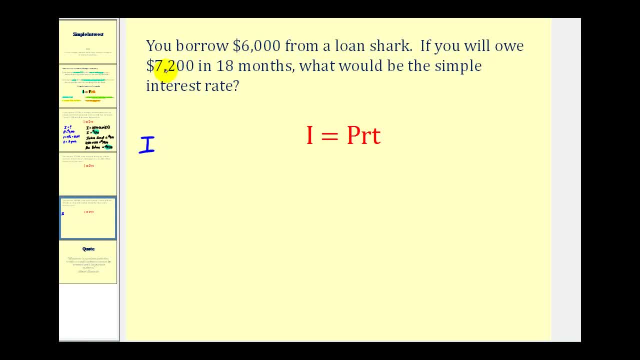 So if you borrowed $6,000, and then you owe $7,200, the difference would represent the amount of interest. So the interest is going to be $7,200 minus $6,000.. So our interest is equal to $1,200.. 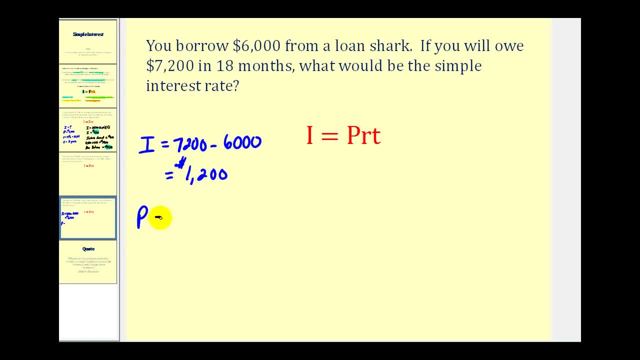 P represents the principal or starting amount. The loan amount was $6,000.. We're trying to solve for the interest rate. Now. our time is 18 months, but remember that the time has to be expressed in years. Well, since 18 months is 12 months plus six months. 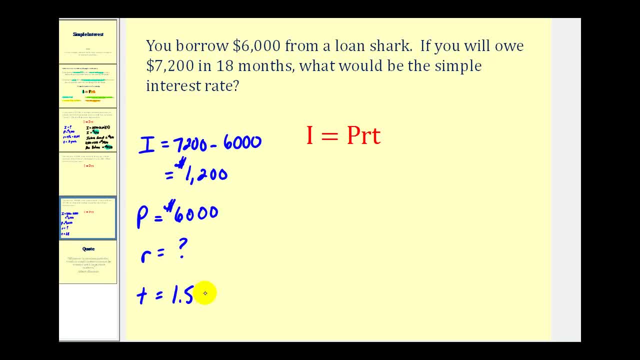 18 months is equal to 1 1⁄2 years or 1.5 years, So it is important that we do have to have our time in terms of years. So let's go ahead and set this up and see if we can solve for R. 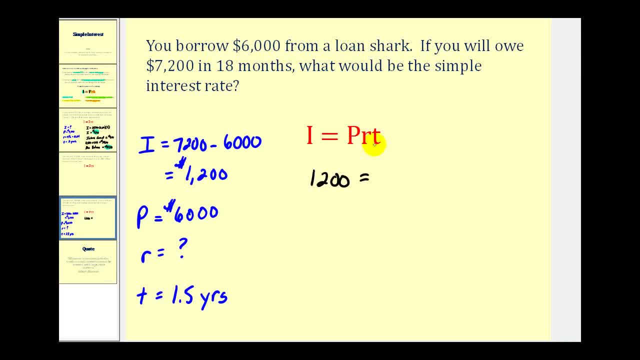 I, which is 1,200, must equal P, which is 6,000, times R, which we're solving for. Let's go ahead and set this up and see if we can solve for R. I, which is 1,200, must equal P, which is 6,000, times R, which we're solving for. 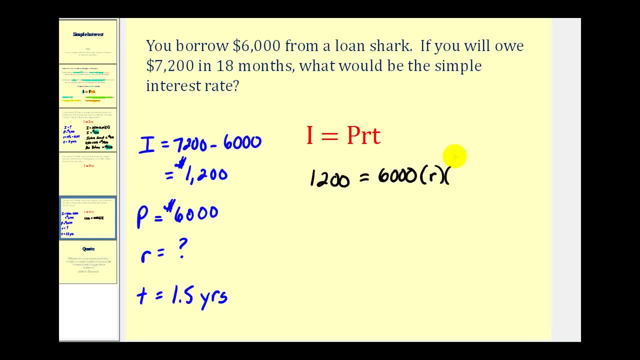 Let's go ahead and set this up and see if we can solve for R I, which is 6,000, times R, which we're solving for times T, which is equal to 1.5 years. Let's go ahead and simplify the right side.